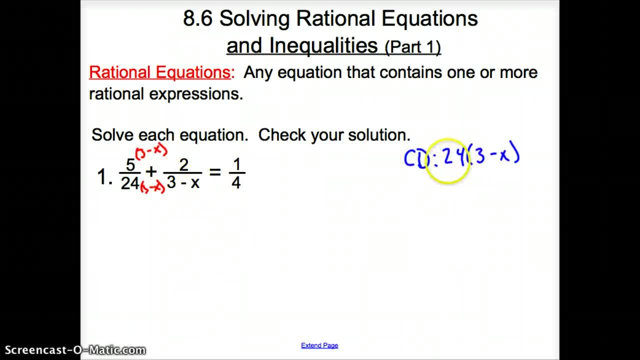 Now, how do I get this 3 minus x to be our common denominator? I need to take that times 24.. So I take that times 24.. Then the 4, what do I need to take that to get to 24?? 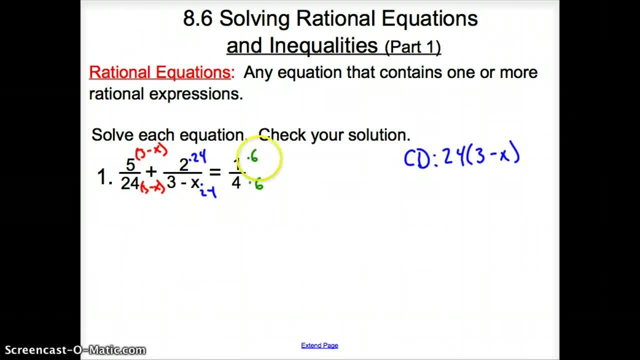 I need to take that times 6,, top and bottom, And then I also need that 3 minus x here and 3 minus x there. Now, when we solve equations, ladies and gentlemen, once you get to the same common denominator, 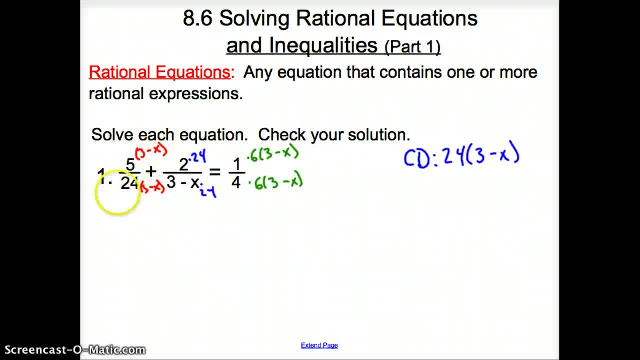 we no longer need that common denominator. So I'm going to write: 5 times 3 minus x, and then that's going to be a plus 24 times 2, and that's going to equal. it's going to equal 1 times 6 times 3,. 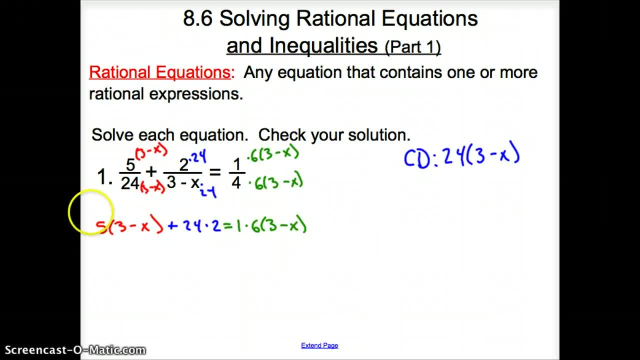 and that's going to equal 1 times 6 times 3 minus x. Once you get here now, it's just like solving any equation that you have seen with x. So let's go ahead and do that. We have 15 minus 5x. 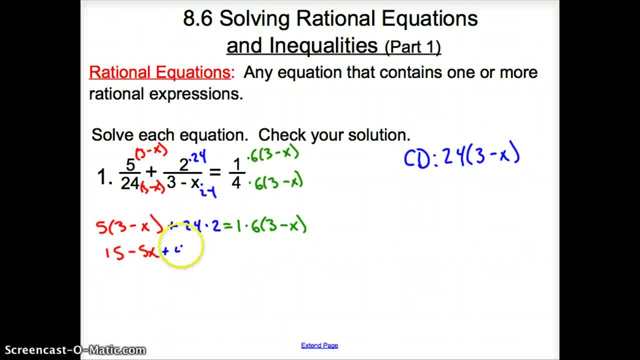 Then we have plus 48, and that's going to equal, and then 1 times. anything is just 1, right? So it's 18 minus 6x. Now, once you get here, we're just solving for x. 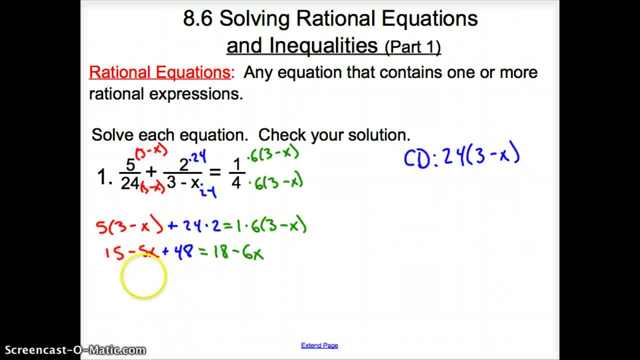 Combine like terms. on this side We have a negative 5x, and then 15 plus 48 is going to be a plus 63. That equals 18 minus 6x. Then I'm adding this x over here, So it's going to be a positive. x plus 63 equals 18, and then I have to subtract the 63 over. 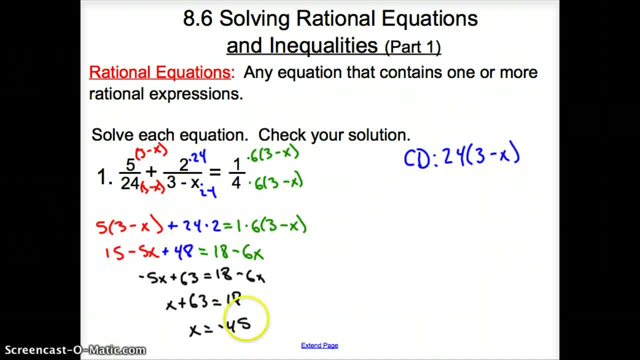 So x equals a negative 45 for our solution. But, ladies and gentlemen, we have to check these answers to make sure they add up, So I'm going to plug in negative 45 in for all my x's. So I have 5 over 24 plus 2,. 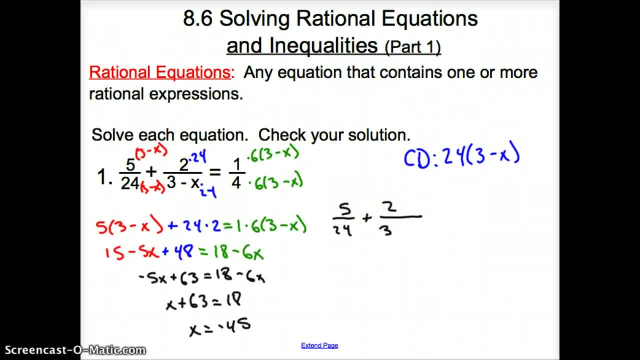 and now that's going to go over 3 minus a negative 45, that equals 1, 4. Well, we have 5 over 24 plus 2 over and then 3, and now it minus a negative turned into a plus. 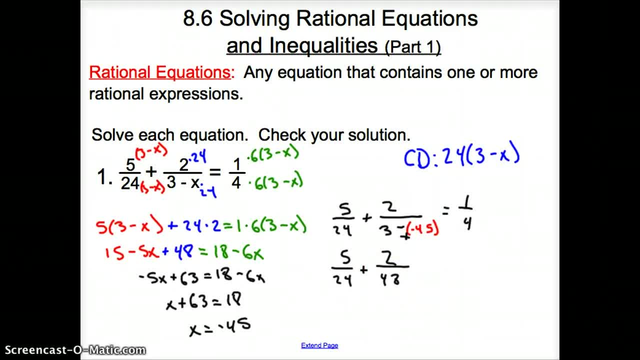 So it's going to be: 2 over 48 equals 1 4th, and now does this add up to 1 4th? It's 1 4th equals 1 4th, so it's good. 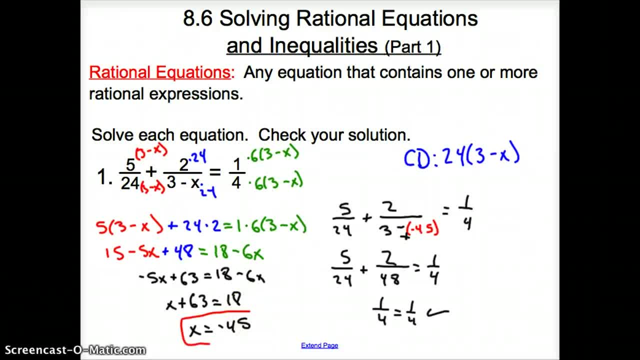 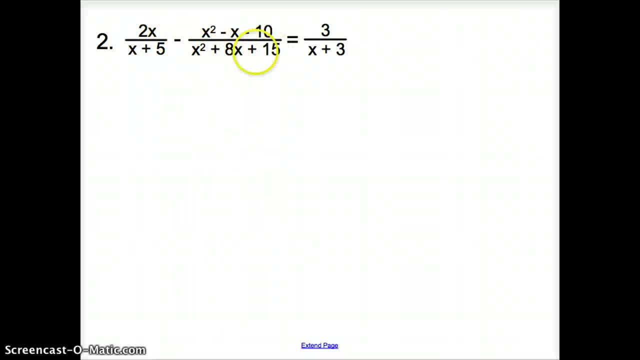 So our answer then checks out: x does equal a negative 45.. Now with number 2, it looks a little bit trickier as we have this polynomial right here. But let's just factor this polynomial So it's going to be x plus 5 and x plus 3, because 3 and 5 multiply to 15 but add up to 8.. 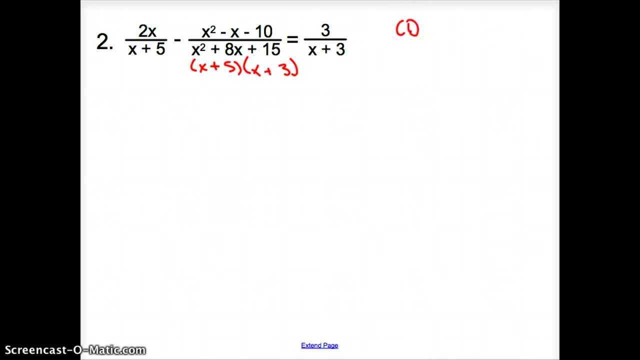 So our common denominator is going to be x plus 5 and x, or times x plus 3.. So here we go. What do I have to get this denominator? what do I have to take times this denominator to get this? Well, that's going to be x plus 3.. 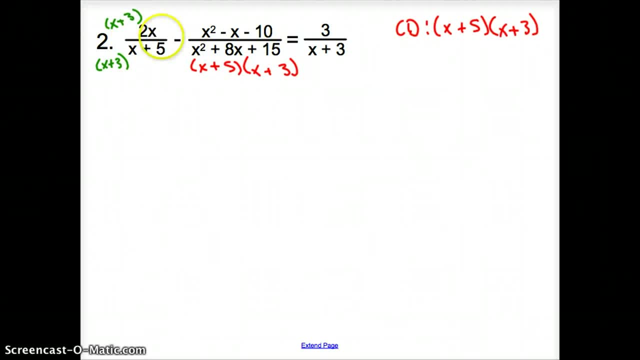 So what you do to the bottom, you have to do to the top. Now this is already at my common denominator, and so then we move on to here. What do I need to multiply this to get that? That's going to be x plus 5.. 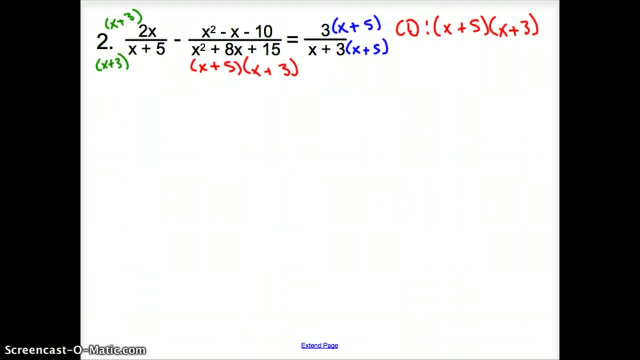 So what did I do to the bottom? I have to do to the top. Once we found the same bottom with equations, ladies and gentlemen. Once we found the same bottom with equations, ladies and gentlemen. Once we found the same bottom with equations, ladies and gentlemen. 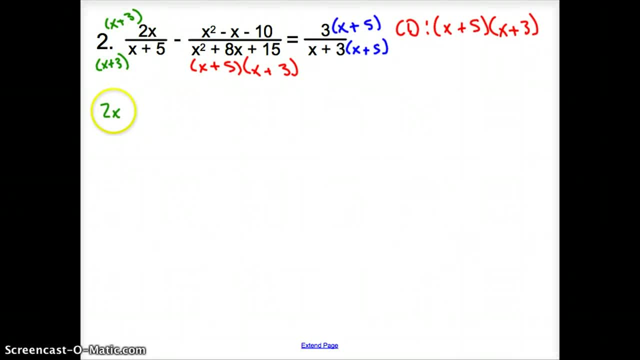 we can just bring it down Here. it's going to be 2x and then x plus 3.. We're just bringing down the top. We're just bringing down the top. Now, be very careful, ladies and gentlemen. This gets a lot of people. 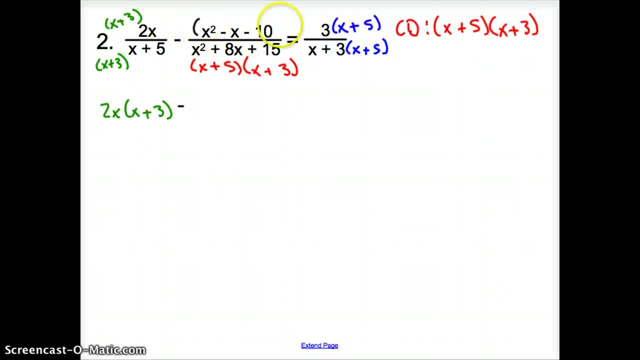 With this minus right here. we have to put this guy in parentheses, So it's going to be a minus x squared minus x minus 10.. We are putting that in parentheses. We are putting that in parentheses. That's going to equal now 3 times x plus 5.. 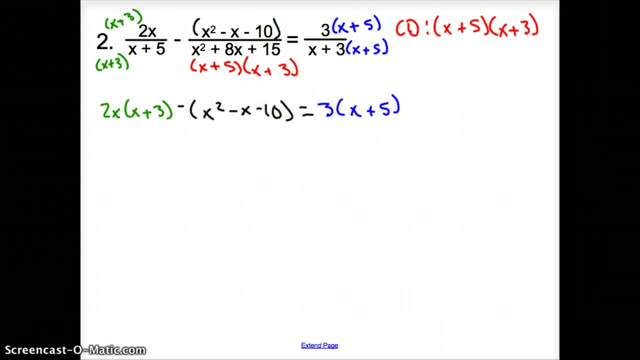 Once we get to this step now we can just simplify like you have been doing. So it's 2x times x, which is a 2x squared plus 6x. Now here's the big reason why we put this in parentheses. 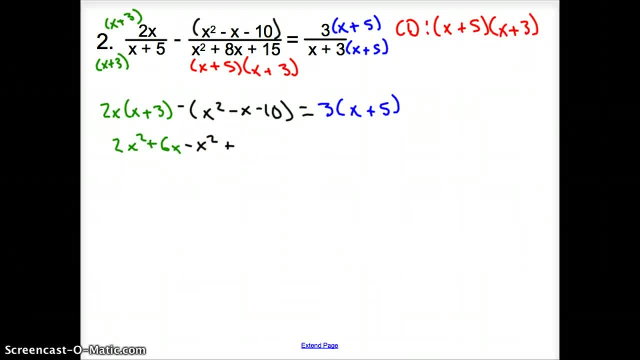 because it's a negative x squared plus x plus 10.. That's going to equal 3x plus 6x. That's going to equal 3x plus 6x. That's going to equal 3x plus 15.. 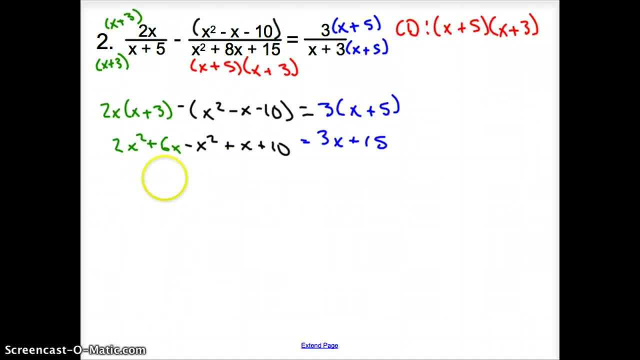 We simplify this side to get an x squared plus 7x plus 10.. That equals 3x plus 15, bringing everything over to the other side Now, it is x squared plus 4x minus 5.. That equals 0.. 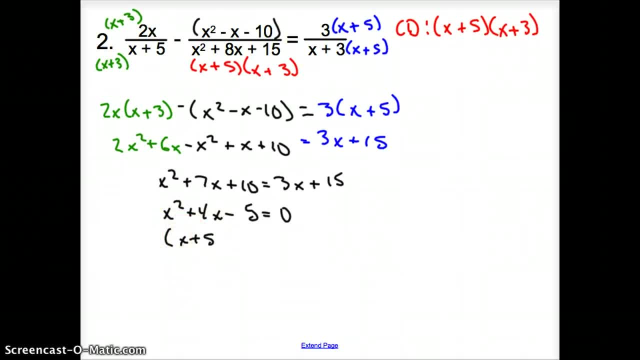 Factor to get x plus 5. Factor to get x plus 5. Factor to get x plus 5.. x minus 1. That equals 0. Here we come up with: x plus 5 equals 0. What else do we have? equals 0?. 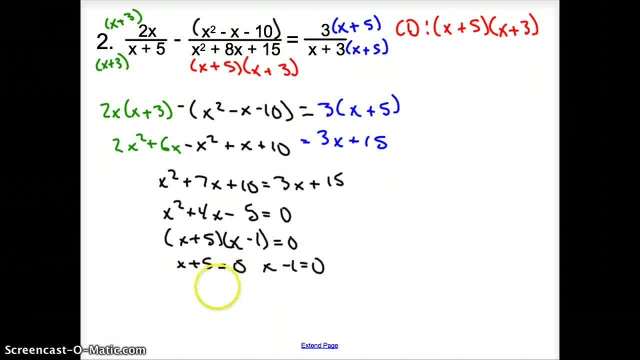 x minus 1 equals 0.. Finally, ladies and gentlemen, we can say that x equals a negative 5 and an x equals 1.. Now, we have to check these. Now, ladies and gentlemen, what we want to do is put in negative 5, in for all your x's. 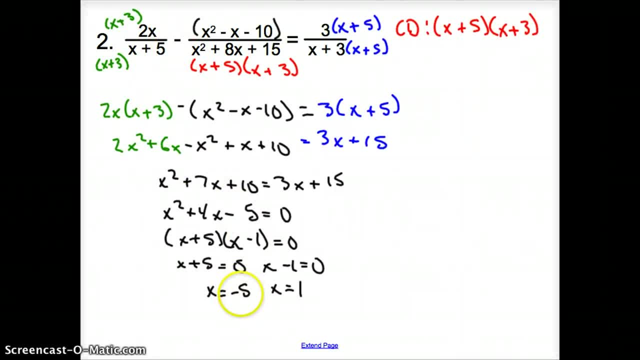 or is there a little bit, A little bit easier way We can put this negative 5 in for that x right on the bottom of the fraction? Well, I have negative 5 plus 5.. That's going to give me 0.. 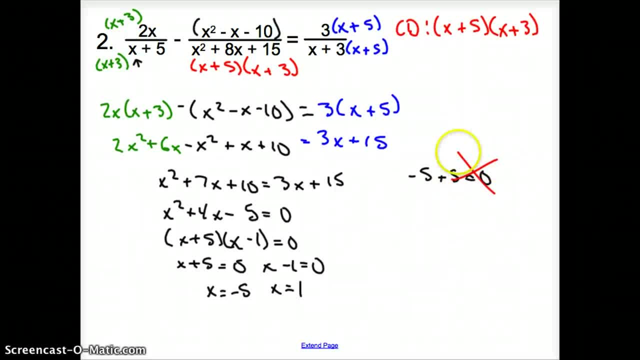 Can I divide by 0?? No, you cannot divide by 0. So, since we put it on the bottom and got 0, we cannot divide or we cannot have negative 5 as our solution. Then we look at 1.. 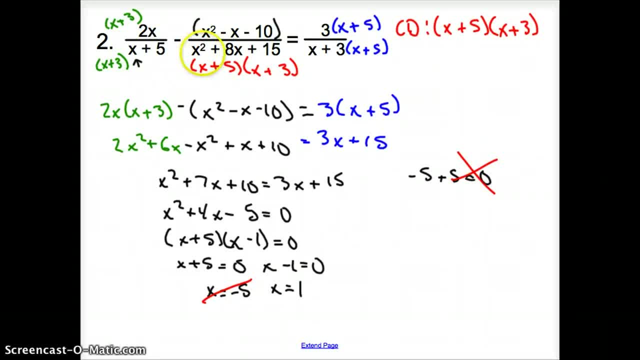 If we put 1 in, does that give me a number, not 0?? Yes, 1 in here and here, not 0, correct, And 1 in here, not 0. So our only answer is now: x equals 1.. 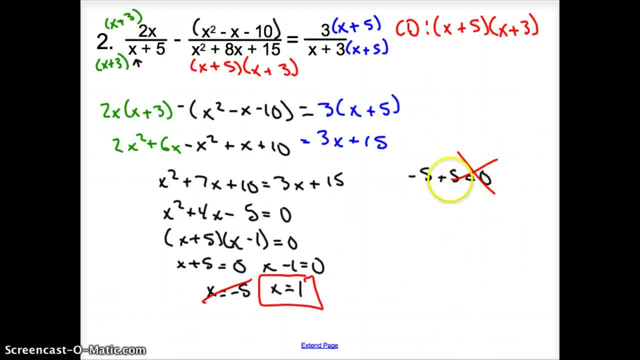 So, ladies and gentlemen, there will be cases where we do not, or we come up with a solution, we check it and that is not in our solution set One more. Here we go Now. look at all the bottoms. 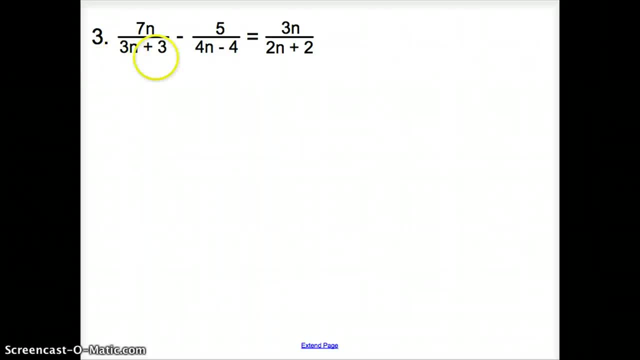 We need to get all those numbers to a common denominator. First thing we have to do is factor. So I factor. I take out A 3 from here to get n plus 1.. Take out a 4 from here to get n minus 1.. 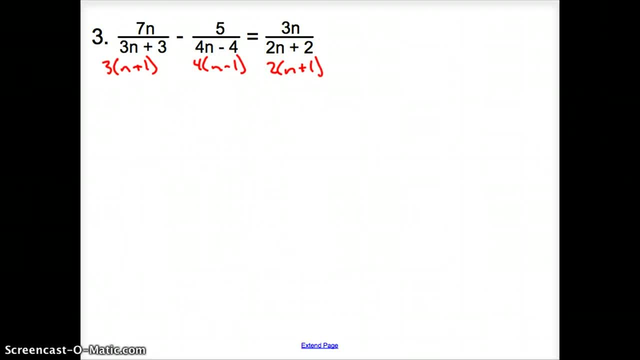 Take out a 2 from here to get n plus 1.. Now we look at all of our factors. Well, what do we have? What's going to be common for our numbers? Multiply them up, They give us 24, but they also multiply to 12,, all of them going to 12.. 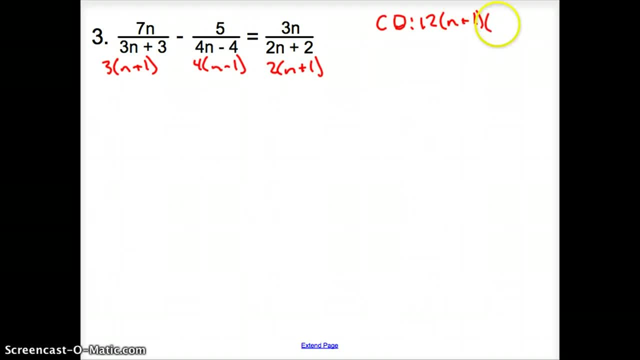 Then our polynomials: We have an n plus 1, and we have an n minus 1.. Looking to get all my denominators to this guy right here. Now, what do I need to take Times that 3 to get 12.. 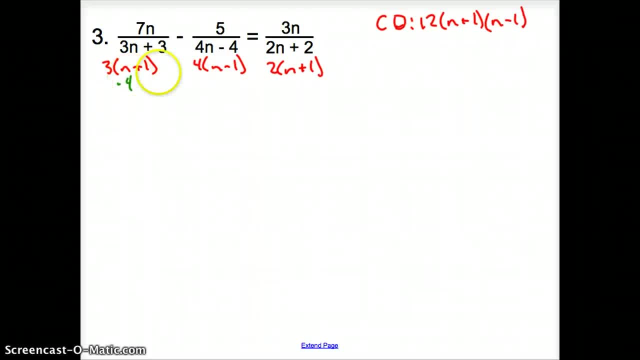 I need to take it times 4.. How about? what am I missing from my polynomials n minus 1.. So I need to take this guy times 4, and n minus 1.. Moving here, what do I need to take the 4 times to get 12?? 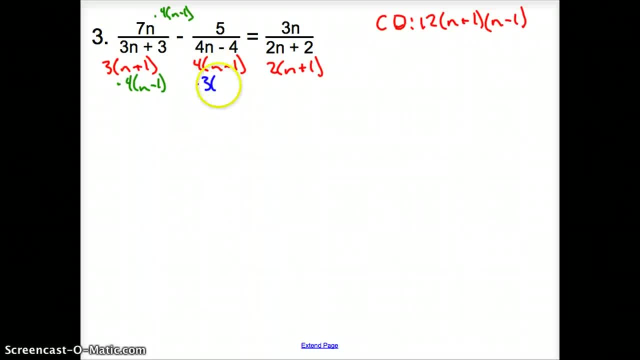 I need to take that times 3, and then I need an n plus n plus 1 for my polynomial. What you do to the bottom, you have to do to the top. And then here, what do I need to take times 2 to get 12?? 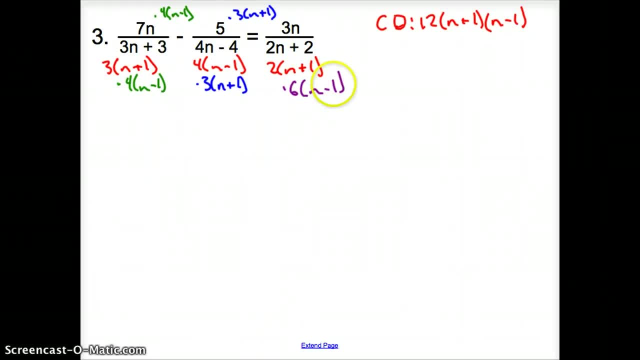 I need to take it times 6, and then I need an n minus 1.. What you do to the bottom, you have to do to the top. So now, once we do that, we're ready to go. So once we have the same common denominator, just drop it and worry about the top. 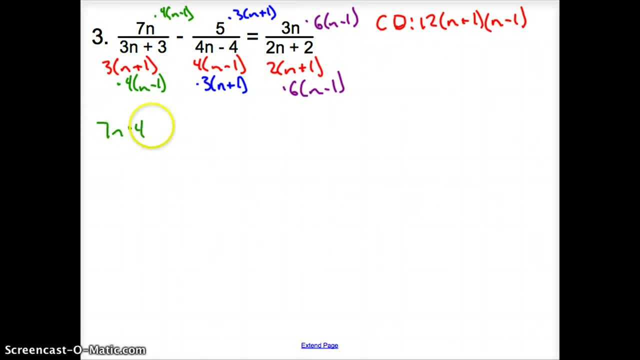 We have 7n 7n times 4, and then n minus 1.. Again, ladies and gentlemen, be very careful with that minus sign. Minus 5 times 3n plus 1. And then that's going to equal 3n times 6, and then n minus 1.. 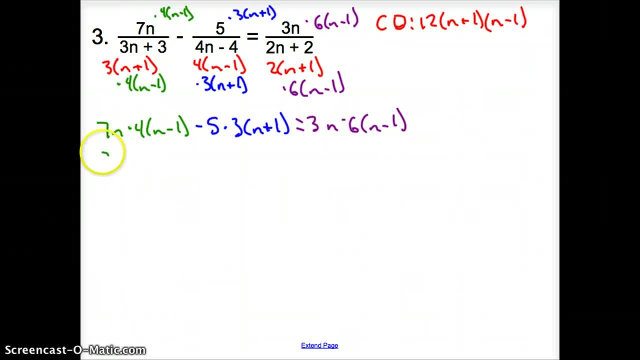 Let's simplify everything. We have a 7n and now I'm going to put- I'm going to distribute this- 4 first. You can take this 7n times 4, not a big deal, but it's going to be 4n minus 4.. 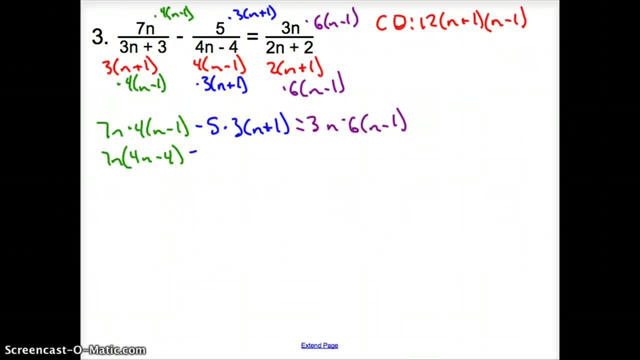 And then we have a minus 5 times 3n plus 3.. And then finally, 3n times 6n minus 6.. Let's continue with this Here. let's distribute everything into those parentheses: It's 28.. 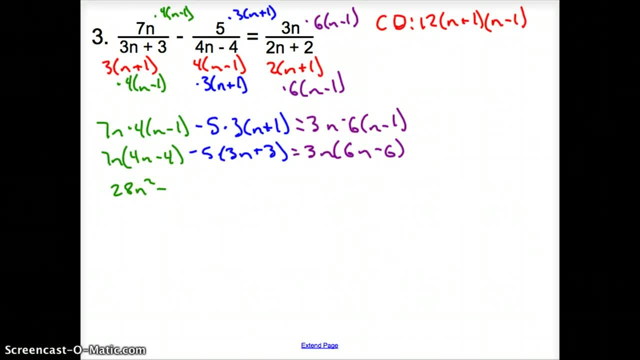 28n squared minus 28n. And then in the blue we have minus 15n minus 15.. That equals 18n squared minus 18n. Clean everything up, ladies and gentlemen. We have 28n squared. 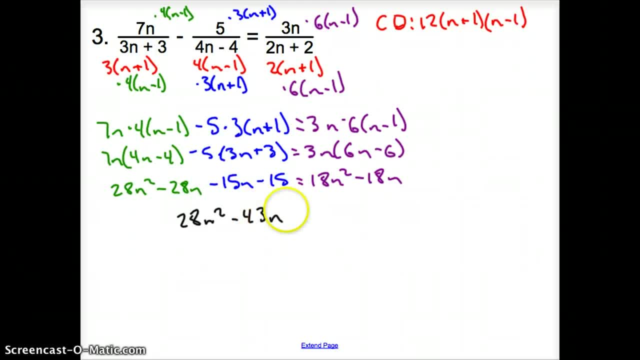 Combining our like terms: Minus 43n, minus 15.. That's going to equal 18n squared minus 18n. Since we have a squared term, we need to get everything to the same side. So I'm going to bring everything over to the left side of the equation. 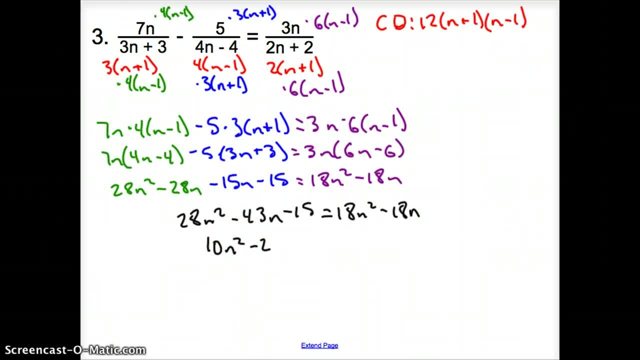 We have 10n squared minus 25n minus 15.. That equals 0.. Now we have to factor this. Yes, you want to multiply first term times the last term. can we factor out anything to make it simpler? Yes, we can. 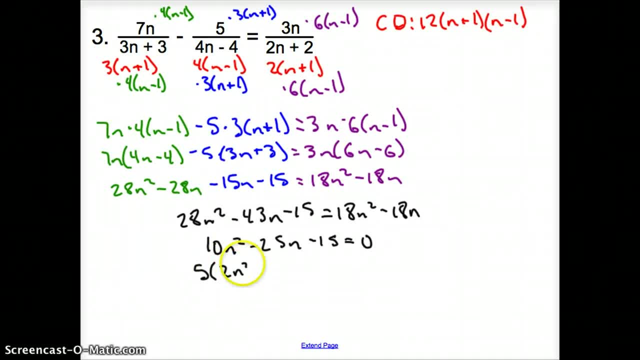 We take out a 5. So we are left with 2n squared minus 5n minus 3. That equals 0. First term times. the last term is negative 6. So we need factors of negative 6 that add up to negative 5.. 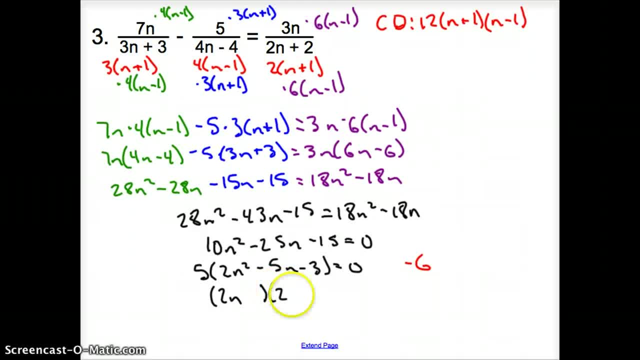 So we bring the 2n down and the 2n down, We have a minus 6.. Minus 6. And a plus 1. We set it equal to 0. We'll close that 0 off. Take a times 5 up front. 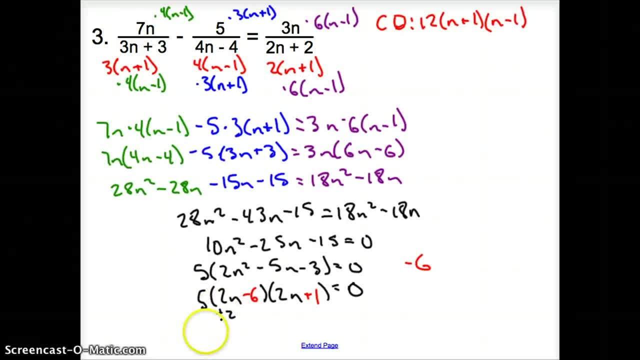 Now we need to take a 2 out right, Because we brought too many 2s down. So it's 5 times n minus 3.. Times 2n plus 1 equals 0. Set these guys. We do not care about the 5.. 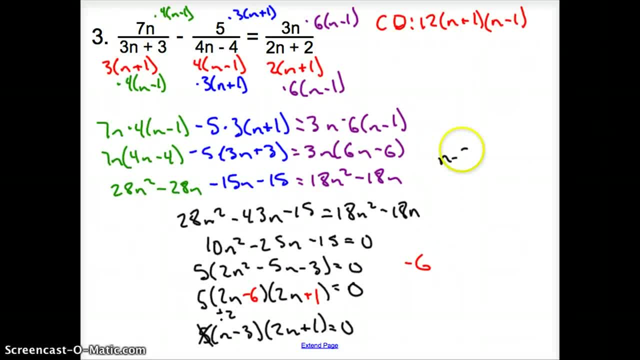 We set these guys equal to 0. So it's going to be n minus 3 equals 0. So we have n equals 3.. And then we have 2n plus 1 equals 0.. Subtract over the 1.. 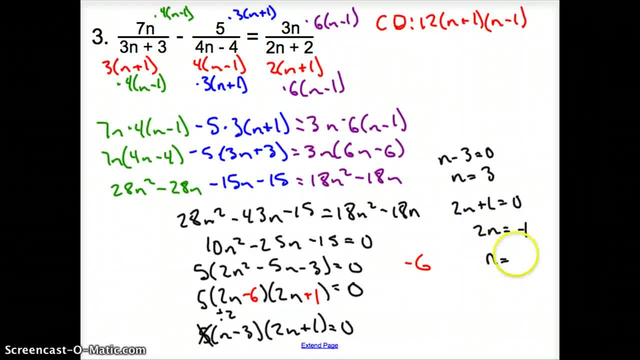 2n equals a negative 1.. Divide by 2. n equals a negative 1 half. Finally, now we go ahead and check the 3. We put it in for just the bottoms. It is positive. It is positive. 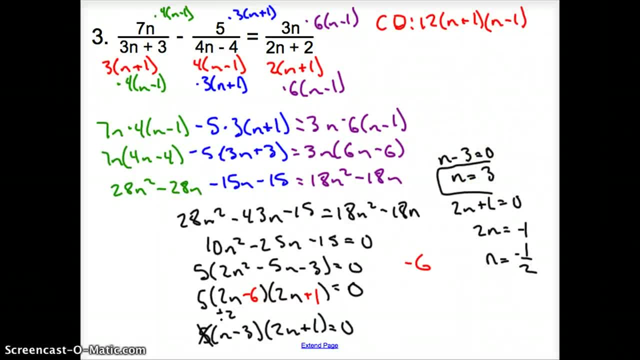 It is positive here, So n does equal 3.. Then we put in 1 half. It is positive, It is not 0 here And it is not 0 here, So n does equal a negative 1 half. So we found both of our solutions. 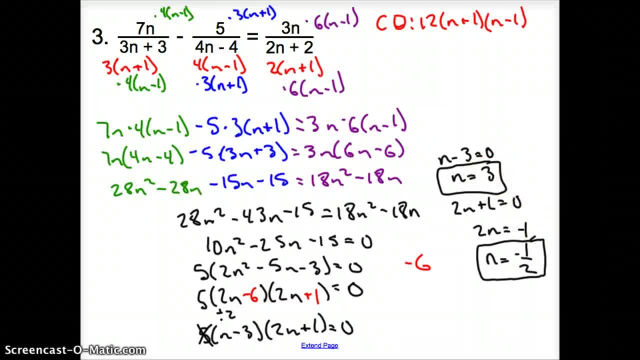 Sometimes you'll have 2 solutions, Sometimes you'll have 1 solution, Sometimes you'll have no solutions, if we check it. Well, ladies and gentlemen, yes, it is a lot of work. Yes, it does check some of your abilities. 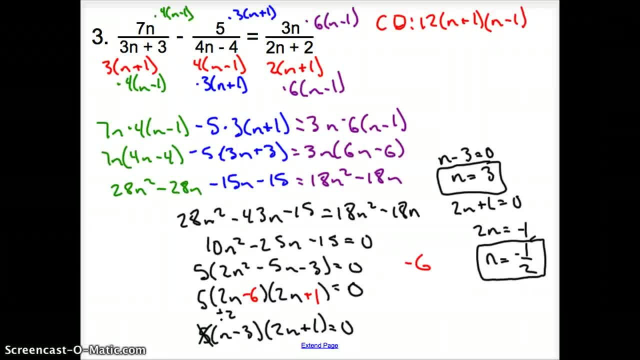 But just hang in there, Go by the process And you will be fine. And that does it for Section 8.6, Solving Rational Equations and Inequalities. Good day. 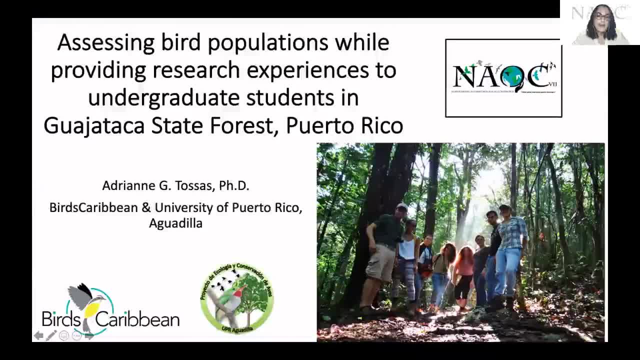 I will be the first presenter in this session. Again, I'm Dr Adrienne Tossos. I work at Birth Caribbean and at the University of Puerto Rico in Aguadilla. The topic of my presentation is assessing birth populations while providing research experiences to undergraduate students. 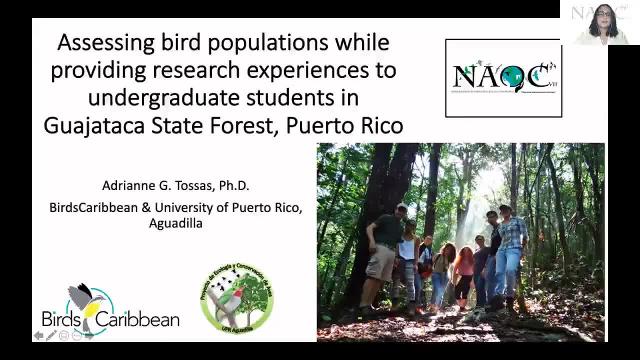 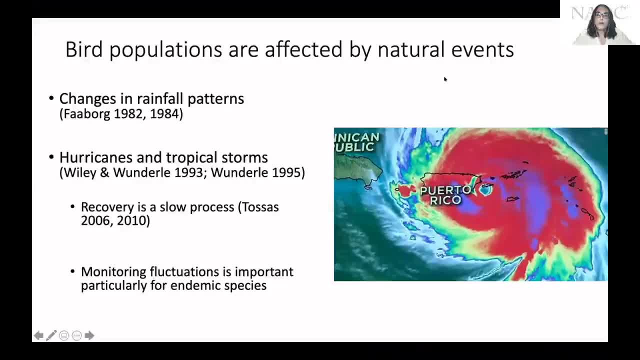 in Oaxaca State Forest, Puerto Rico. Birth populations are affected by natural events. This has been shown before when hurricanes have passed through the region, particularly by the work done by Wonderly after the Hurricane Hugo in 1989.. We know that the effects of hurricanes can.